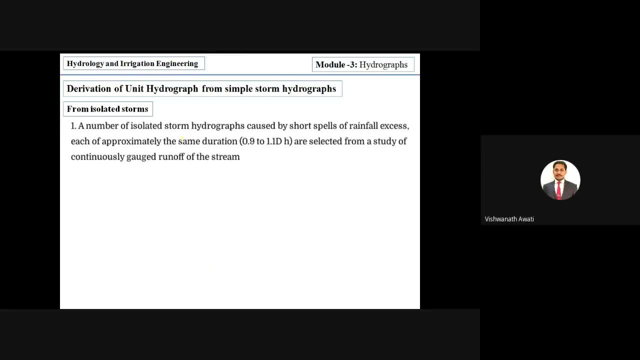 some simple steps, right. So first step is the number of isolated strong hydrograph caused by short spell of rainfall axis, each of approximately the same duration. So we are collecting the data of isolated strong hydrographs and of different isolated hydrograph, but the, if you take the duration of time, it is 0.9 to 1.1 duration. 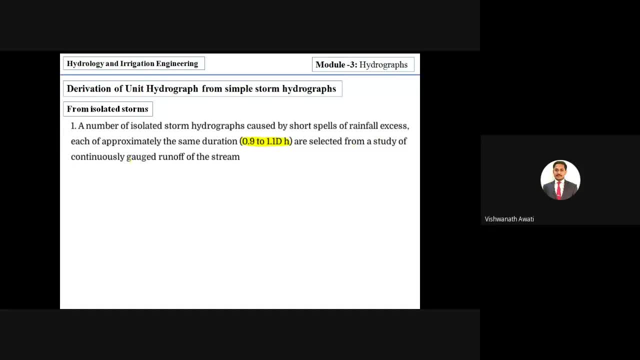 are right, are selected from the study of continuously gauged runoff. So continuously monitored gauged runoff data will be collected right So, but at the flood hydrograph using analysis should be selected so as to meet them following desirable features with respect to the 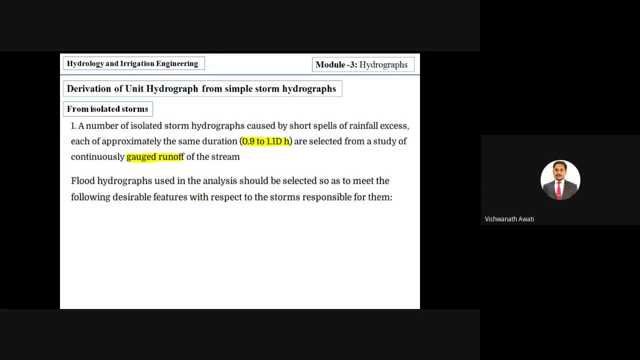 storms responsible for them. So here it is what we have to consider: Desirable features of hydrographs which we are using for analysis. So we have a different desirable features requirement. first one is: the storm should be isolated. storm occurring individually- right, it should be individually occurring. Next is the rainfall should 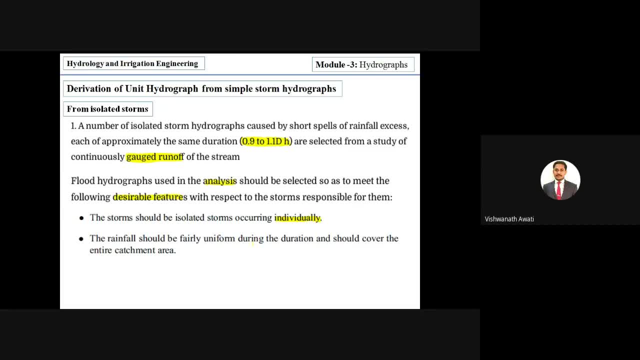 be fairly uniform during the duration and should cover in the entire catchment right. the rainfall should be fairly uniform during the entire duration and it will be for entire catchment. Next is the duration of rainfall should be one-fifth to one-third of the base log. The rainfall axis of the selected storm should be. 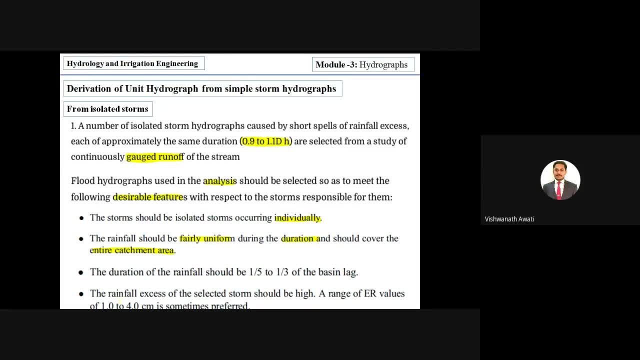 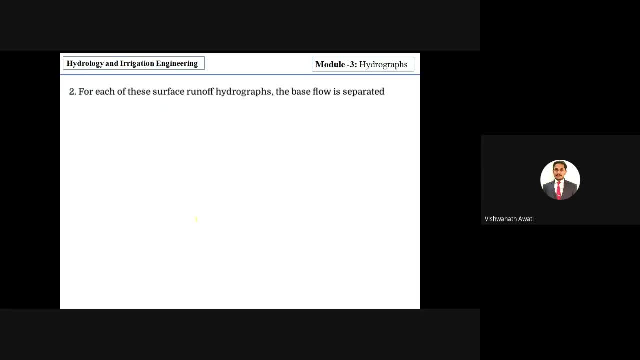 higher, the higher in the range of 1 to 4 centimeter. Next is after getting the flood hydrograph right, so we have to make the next step right. When we want to make the derivation of unit hydrograph, then we have to get direct runoff hydrograph. So to get the direct runoff. 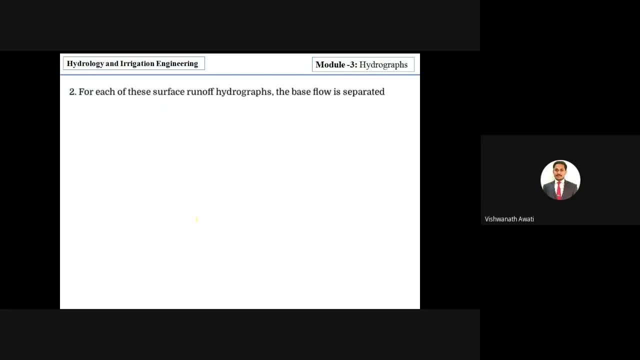 hydrograph, what we have to make The base flow separation from the flood hydrograph. So then we have to go for. next step is base flow separation and we have a three method and you can use any one method. Next is, after the base flow separation, we will get direct runoff hydrograph. 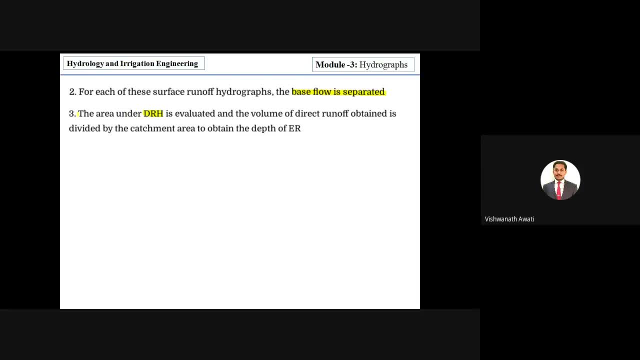 and from this direct runoff hydrograph we can make the area calculation of unit hydrograph. Then, after the area calculation of unit hydrograph, then we can calculate volume of direct runoff obtained right. We can calculate the volume of direct runoff and that volume of direct runoff is divided by catchment. 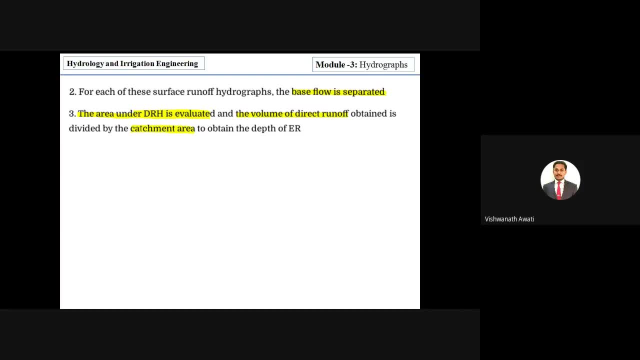 area. Why it is Because there is an assumption that area under the direct, the area under the direct runoff hydrograph, is equal to the unit depth of catchment area, the unit excess rainfall. and it is an assumption and from that we can make the evaluation and you can calculate the excess rainfall right, And we will see this. 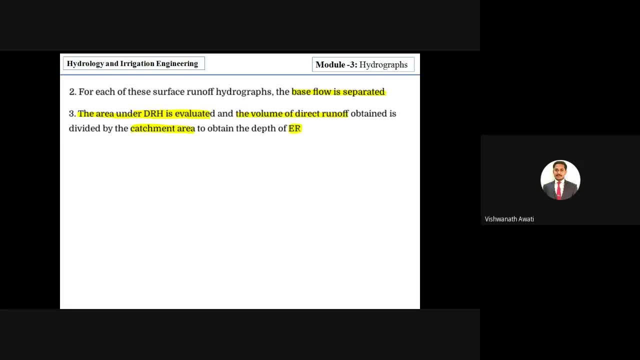 condition when we solve the problem that you can easily understand how we are making the excess rainfall calculation from catchment area and volume of direct runoff right. okay, So then the ordinates of the various direct runoff are divided by the respect to excess. 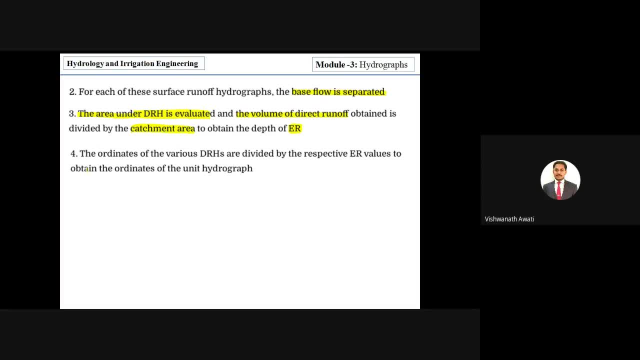 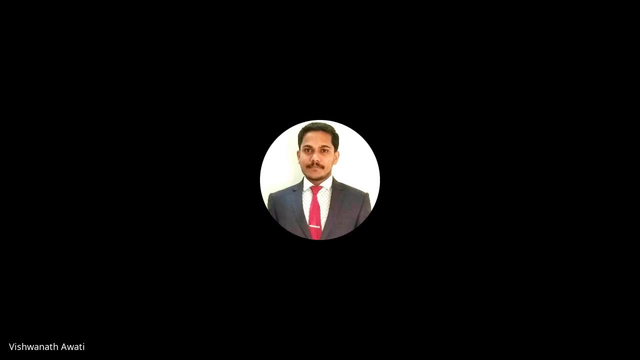 rainfall values to obtain the ordinates of unit hydrograph. So these four steps are very important to solve the problems. So our main intention is to derive ordinates of unit hydrograph. To get ordinates of unit hydrograph we require ordinates of direct runoff hydrograph right. 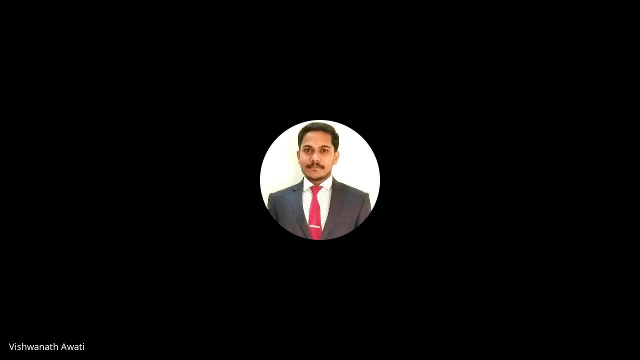 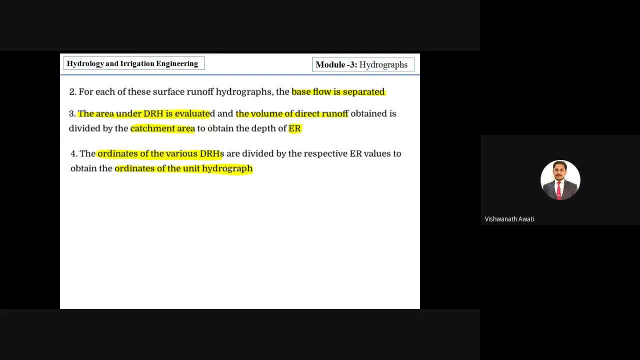 How to get the ordinates of direct runoff By Bayes plus operation correct. So then, how to get the ordinates of unit hydrograph? By dividing ordinates of the various direct right, dividing excess rainfall of excess rainfall and dividing the ordinaires of direct runoff. 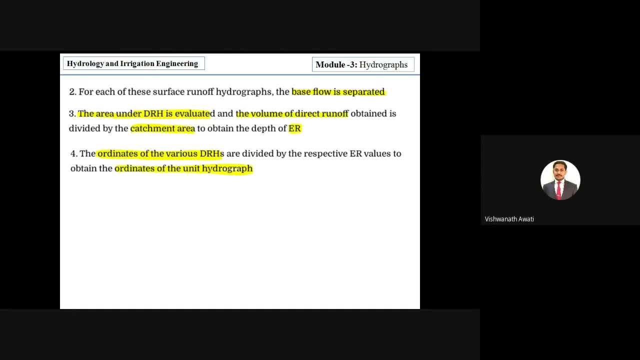 hydrograph. we will get ordinaires of unit hydrograph and this part we will understand when we solve the problem. Next is, after getting ordinaires of unit hydrograph, we can make the plot. the number of unit hydrograph of the given duration are derived as mentioned the above. 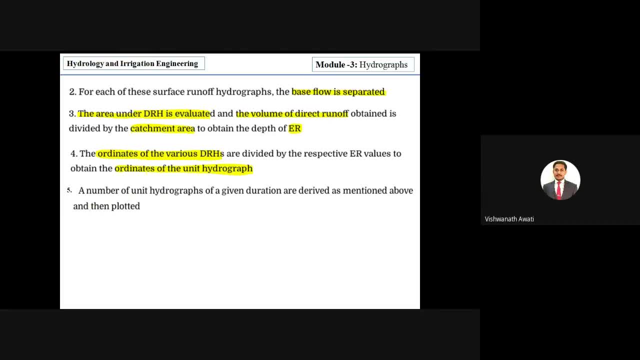 then plotted. after getting the ordinaires, we can make the plotting of different unit hydrographs right. So but the condition here? it is due to the variations, the variations in terms of spatial variation and temporal variation in the rainfall, and due to the deviation of the 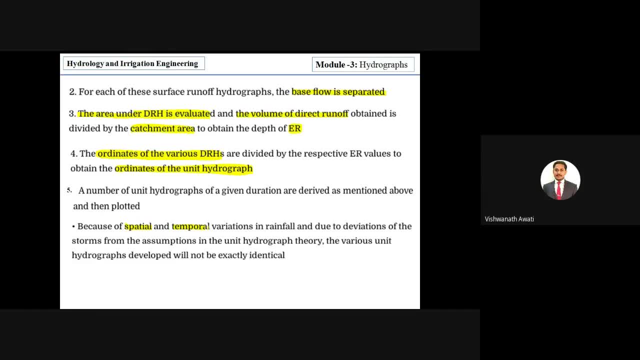 strong from the assumption. in the unit hydrograph theory There is a deviation of assumption and, due to this, the various unit hydrograph developed will not be exactly identical. right, when we are getting a unit hydrograph by these methods, that these are not identical. Why these are not identical? Because of deviations. right, and we will see how to make them best. 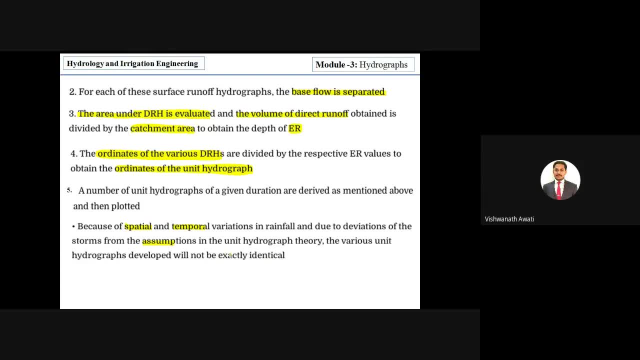 derivation of unit hydrograph in deviation. unit hydrograph Next is: in general, the mean of these curve is adopted when we are not getting exactly identical right because of the deviation from the assumptions of unit hydrograph theory and the variation in the spatial and temporal variation. 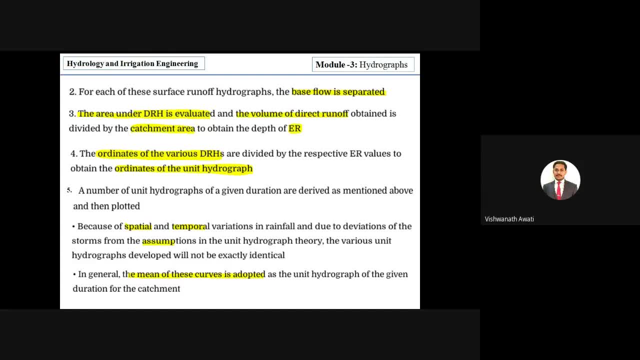 of these curve is adopted as a unit hydrograph of the given duration for of the catchment. for the catchment, then the average of peak flow and the time to peak peaks are computed first. so here it is the peak flow. peak flow and time to the peak flow are computed first right, then then the mean. 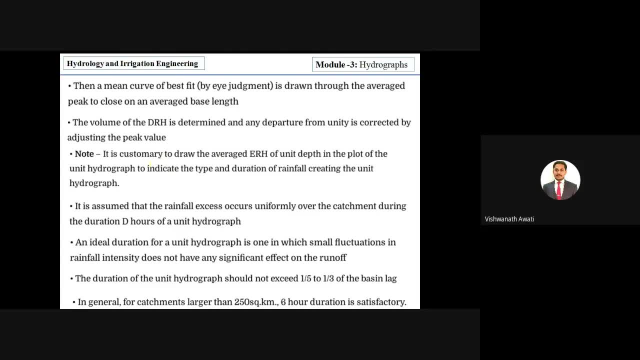 the mean curve of best fit. when we are not getting identical unit hydrograph, then the mean curve of the best fit by i judgment is drawn, is drawn, then the volume of direction of is determined and any departure from the unit unity is corrected by adjusting the peak values. then, as i told there, 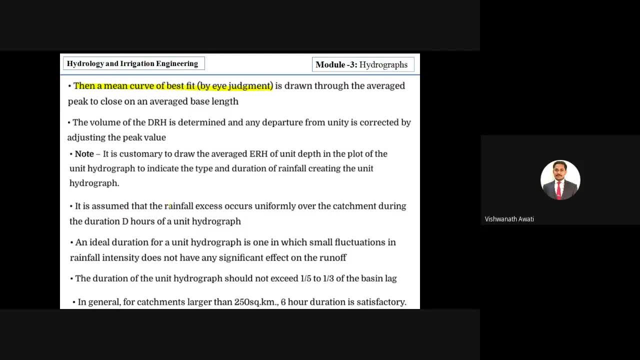 is the assumptions right? that assumptions what we discussed earlier. the same assumptions are that rainfall access occurring uniformly over the catchment during the duration dr. here it is what rainfall access occurring uniformly over the catchment during the duration of the unit hydrograph right. so then the identical. 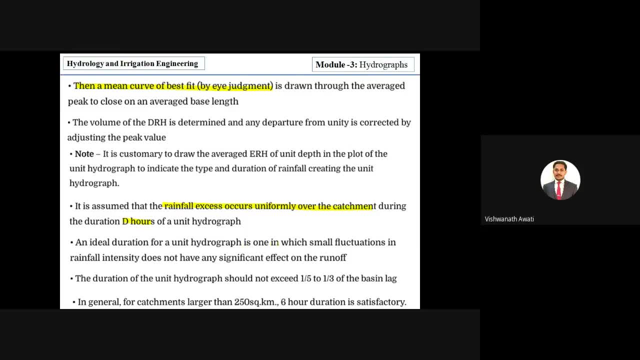 duration for a unit hydrograph is one in which the small fluctuations in rainfall intensity does not have any significant effect on the runoff, then the duration of unit hydrograph should not exceed one-fifth to one-third of the base log, one-fifth to one-third of base log in general for the 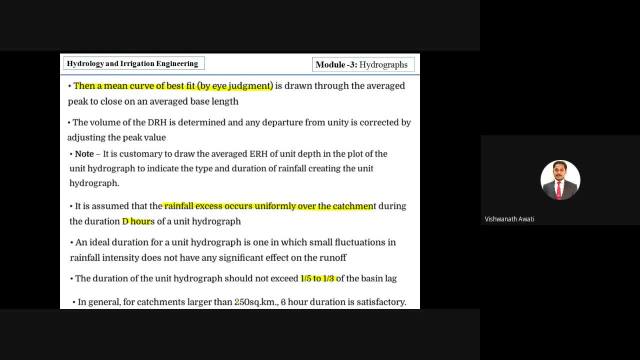 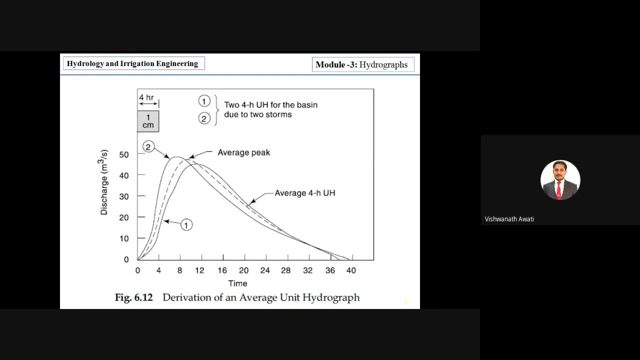 catchments larger than 250 square kilometer. six hour duration is satisfactory, correct. so then we will see the hydrographs. so here, after the derivation right, we have a main steps right. first one: we have to get the collection of data of flood hydrograph, isolated flood hydrographs right. 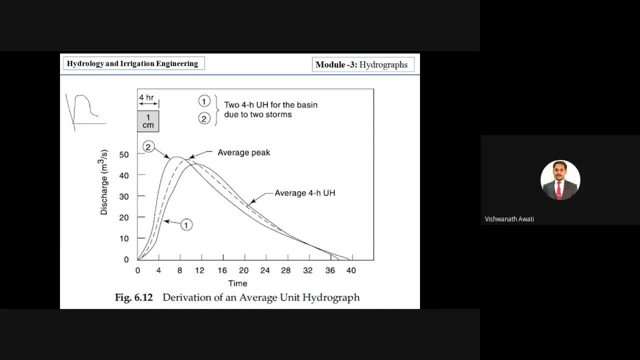 we have to make the first drawing of flood hydrograph. then we have to make the base flow separation. after the base flow suppression we are getting direct runoff hydrograph. from this we can make the volume calculation of direct runoff hydrograph. then that volume is divided by area. 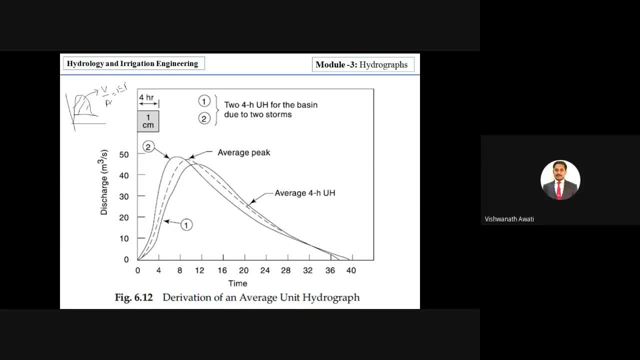 right, then we will get excess rainfall, correct excess rainfall and this excess rainfall are again divided up to each ordinance of director. now, then we will get the ordinance of unit hydrograph. so if we backgammon after returning these unit hydrograph, we will get number of unit hydrographs. 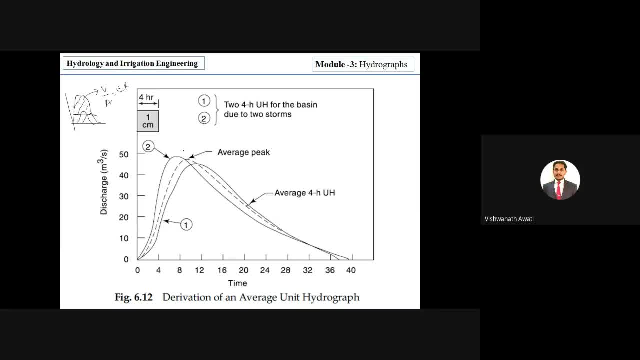 and these unit hydrograph are not identical. you can see, here it is um. do we have a second? here it is one second for our unit hydrograph. again for our units. you can see, here it is not identical, right, because we have a four unit hydrograph, four, our unit hydrograph of different. 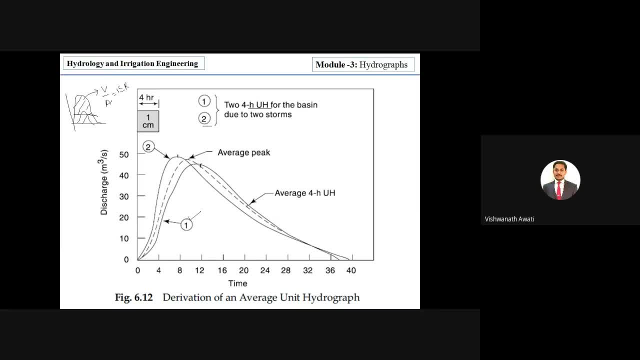 durations a different strong. so here is a unit for our regenerative growth of one parasitics menstruuem generation potential, and four are- and we are makinggenommen bait pads- unit hydrograph of another strong right, but these are not identical. then what we have to do 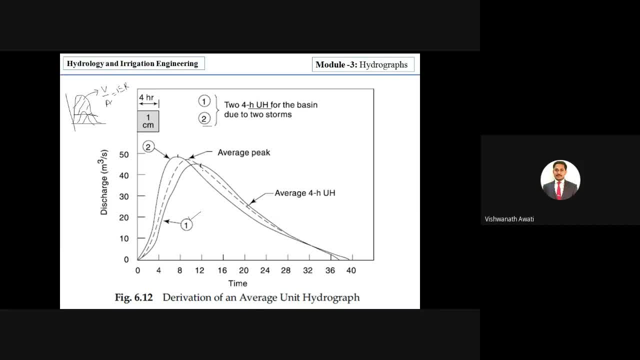 we have to make the best fit of the curve right by eye judgment. right after that we are getting average 4 hour unit hydrograph- average 4 hour unit hydrograph. then peak value is calculated. here you can see peak value is calculated and time per peak value is calculated first. 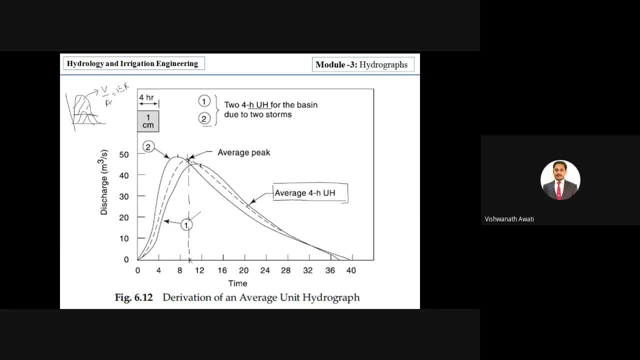 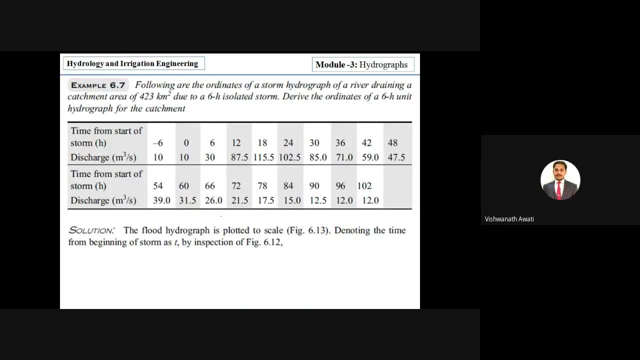 time per peak value is calculated first. then we will solve the one problem and we will understand how to make the derivation of unit hydrograph from the flood hydrograph. so here the in the problem they have given some data right. so here the following are the ordinates of strong hydrograph: 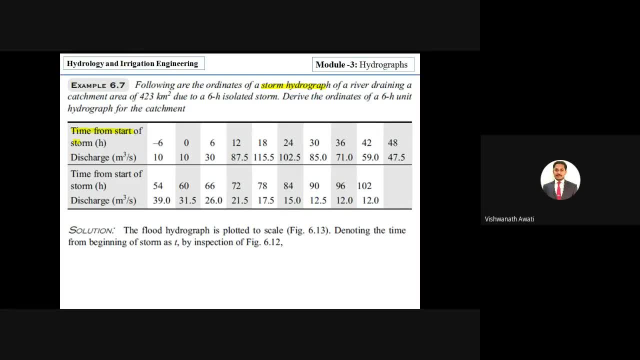 right. they have given ordinates of strong hydrograph with respect to time and discharge of a river, of a river, of a river drain draining storm hydrograph of a river draining catchment area: the catchment area, they have given 420 kilometer square due to 6 hour isolated storm right, the only one storm. 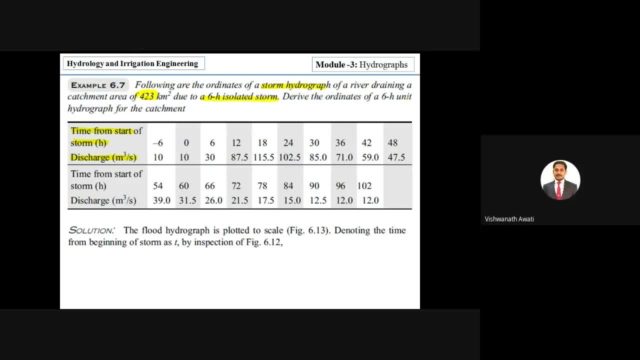 the derived ordinate derive the ordinates of 6 hour unit hydrograph for the catchment. our main concern is 6 hour unit hydrograph. we have to make the derivation right, so then we will see how to solve this problem. i will repeat: they have given ordinate hydrograph of a river draining. 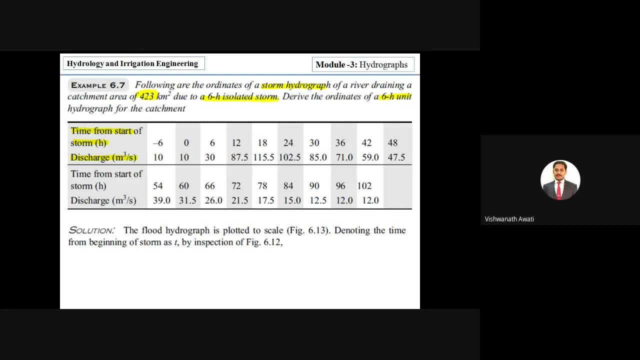 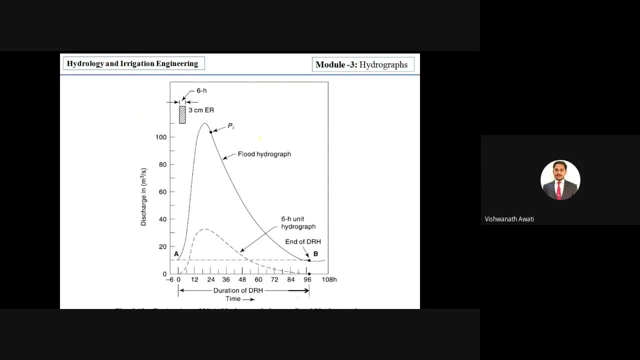 storm hydrograph of a river draining and they have given catchment area and we have to make the 6 hour unit hydrograph derivation from the flood hydrograph correct. so then, first we have to make the plot of hydrograph right. you can see here it is a plot of hydrograph right. so how to draw this flood hydrograph? 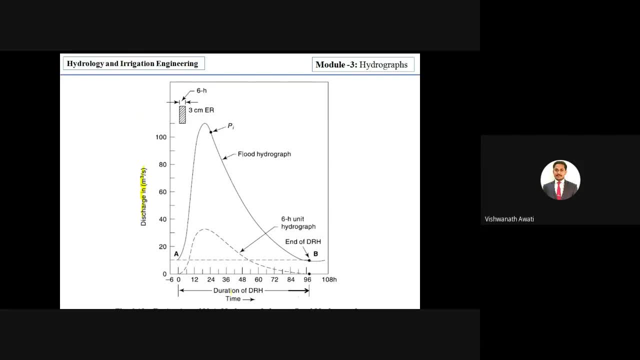 they have given discharge values and with respect to time. so then we will get this height of flood hydrograph. then next step is base flow separation- right? so we have a three method in that first one is a straight line method, right? so here you can see they have used. 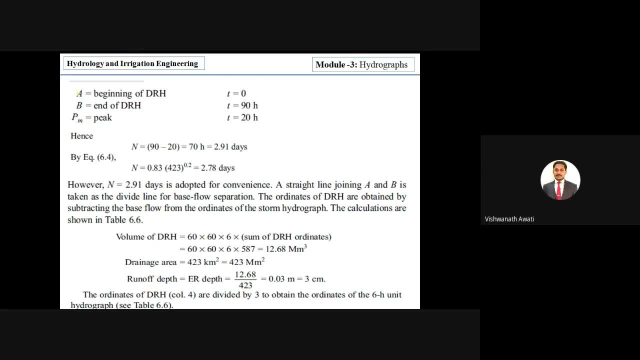 different method. i have taken this from textbook and here they have two method: one with a peak value and peak time. right, so here it is. a is a beginning point of direct run of hydrograph, and the time at the beginning is 0, and b is the end of the direct run of hydrograph and time is a. 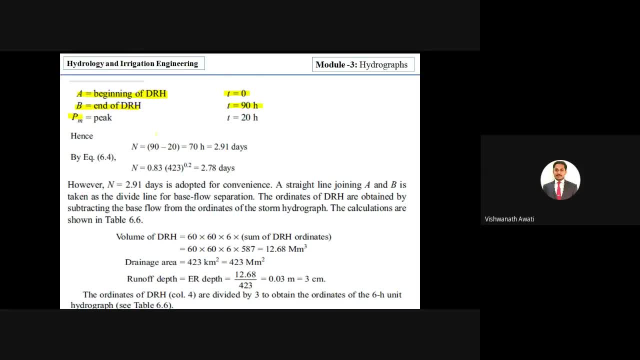 90 hours and p time is 20 hours. so when you get a difference between beginning and end, we will get that n days in terms of 70 hours and it is counted in today it is 2.91 and one more method is we have one more method, is it? 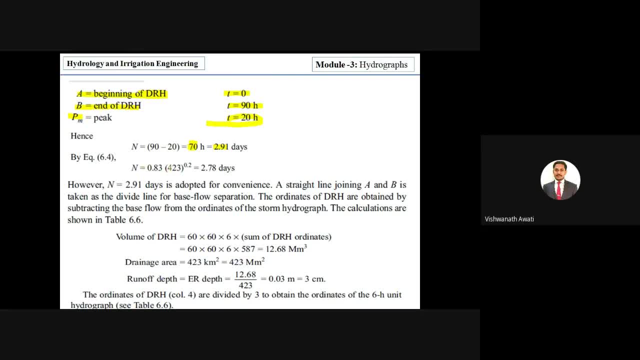 is what we studied: n, equal to 0.83, into catchment area to the power 0.2. so then, after this, this area is given 424, 23 kilometer square, then we will get 2., 2.78 days right. in terms of days, however, n is equal to 2.9 days is adopted for convenience by: 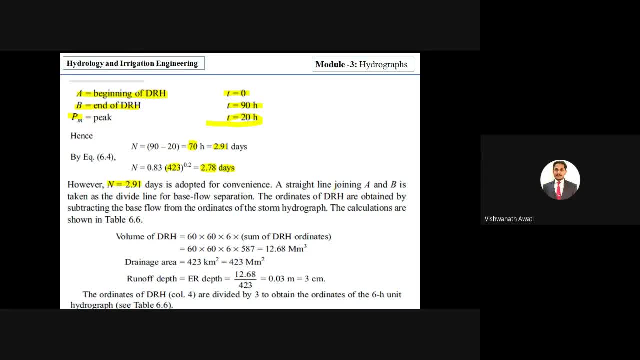 the convenience higher value is adopted. the straight line joining a and b is taken as the divide line for base flow separation. the line of a- b is considered as a divider between direct run of hydrograph and base flow. base flow right, the ordinary of direct run of hydrograph, are obtained by subtracting the base flow from the ordinaires. 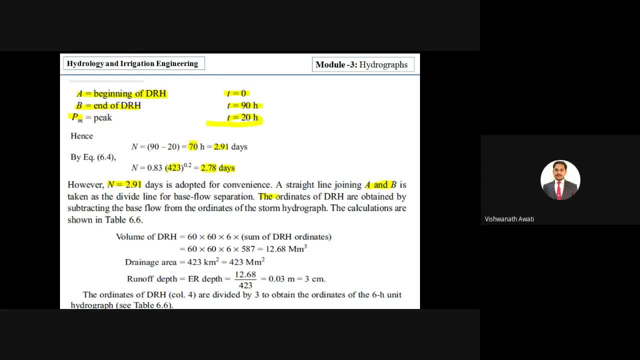 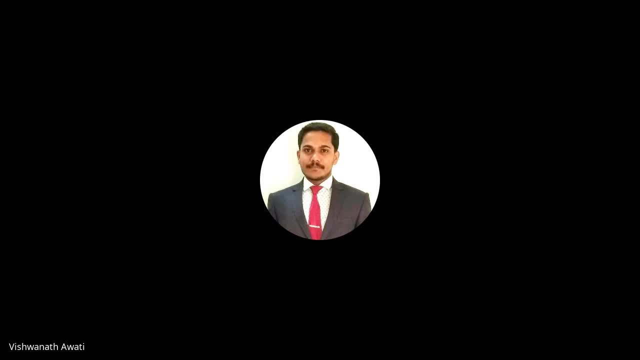 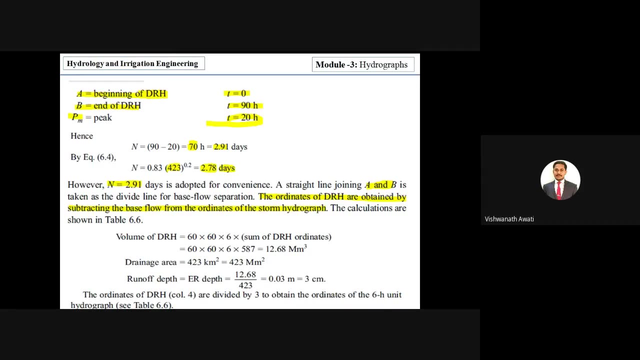 of that storm momento graph. this sentence is very important. so how we are getting the ordinaires of direct run of H quase divisible by this consideration? that is what the ordinaires of direct and now hydrograph are obtained by subtracting the base flow from the ordinaires of the strong hydrograph. so here will get the 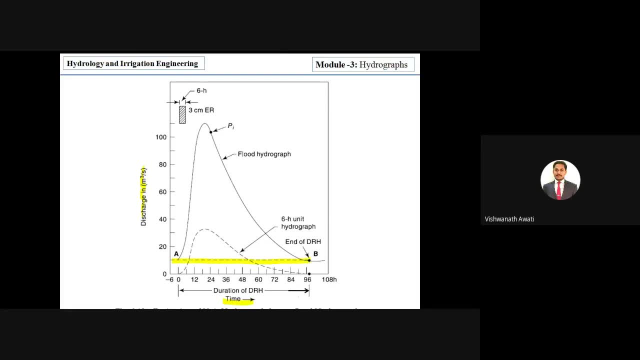 base flow values and you could draw there pedograph and when you join this a, b after the calculation of n days, right, we will get this base flow and from this we will get the value of base flow right. It may be constant or it may be varying. 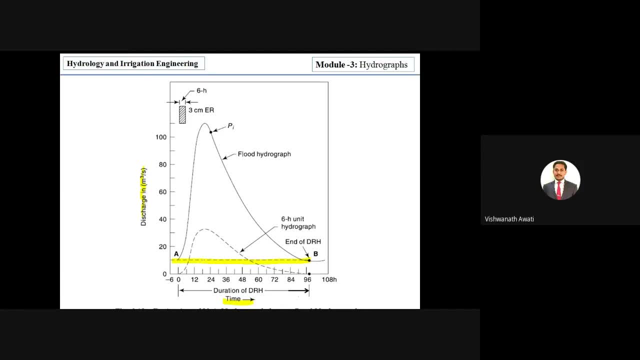 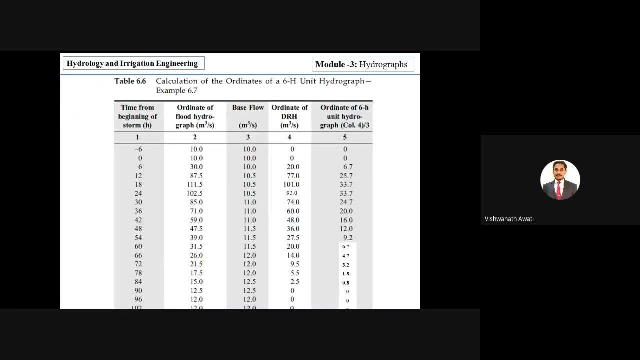 with respect to time also, right. We will see how they are varying with respect to time of base flow, right? So then we will go through the calculation first, then we will go for again remaining calculation. So here we are making the calculation of ordinates of 6 r unit hydrograph. 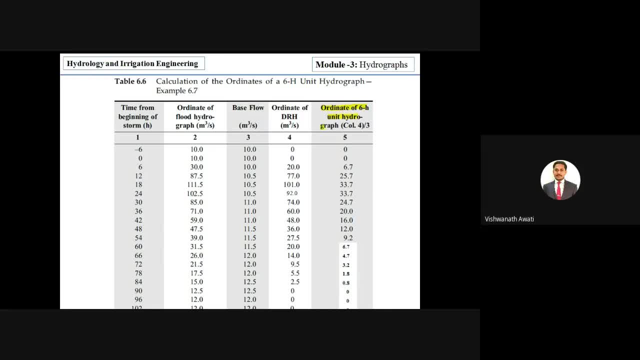 Our main intention is we have to get ordinates of 6 r unit hydrograph, and to get this we have to obtain ordinates of direct runoff hydrograph, and to get this we require base flow, and for this we have to make the base flow separation from the flood hydrograph right. So here, first column, 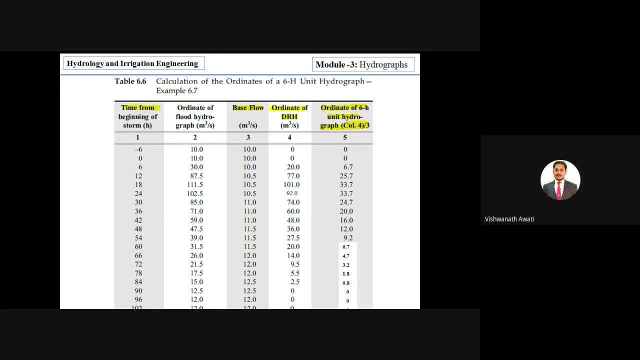 we have to write down time, which are given in the problem. Next, we have to write the down ordinates, which are given in the problem. Next step is, after the drawing the flood hydrograph, you have to make base flow separation. and after the making base flow separation, you will get these: 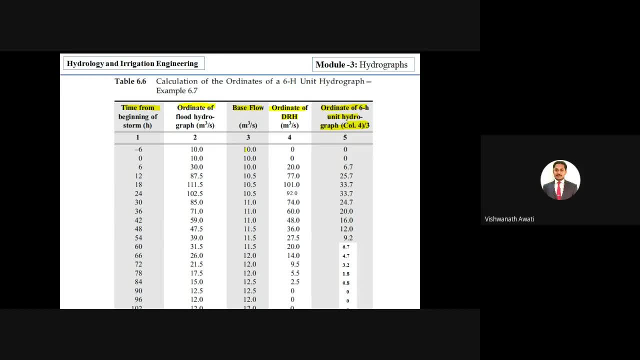 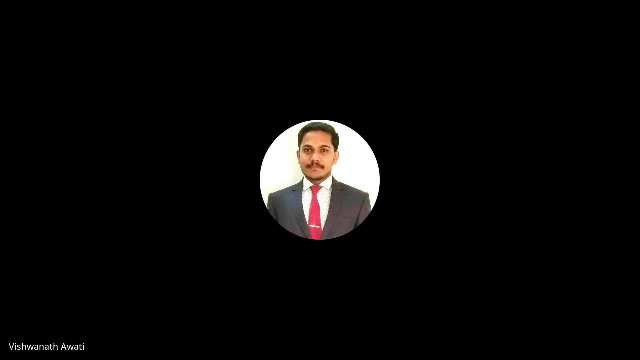 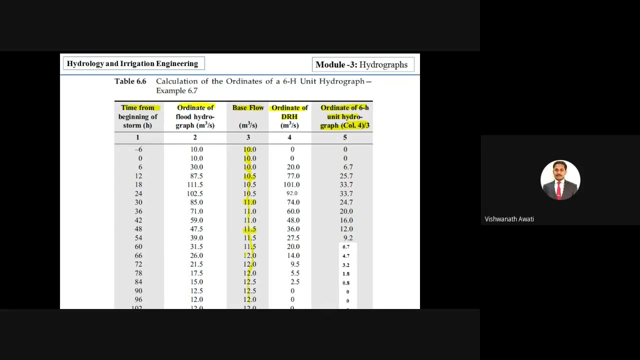 values. As I told, it may be uniform, based on the graph, and it may be changing. So here in this textbook we have taken 10 initially, then it changed to 10.5, again it changed to 11 and again it is changed to 11.5. it is changed to 12, again it is changed to 12.5. right, it will get from the. 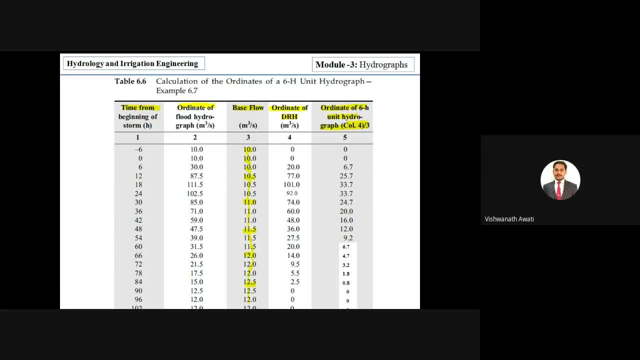 graph. Then we have to make, we have to get ordinates of director and of hydrograph by subtracting base flow from the ordinates of flood. hydrograph means we will get a column 4 by making 2 minus a subtracting column 2 from right, 3, right. So first one is 10 minus 10, 0. 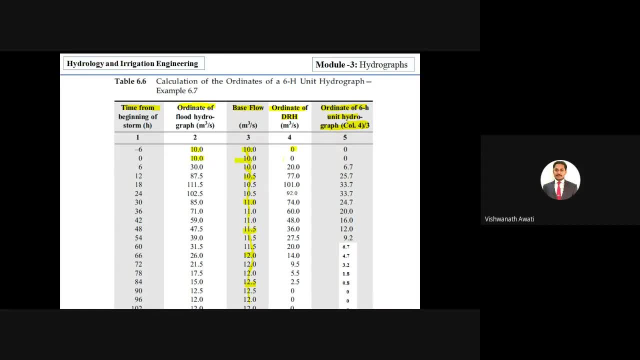 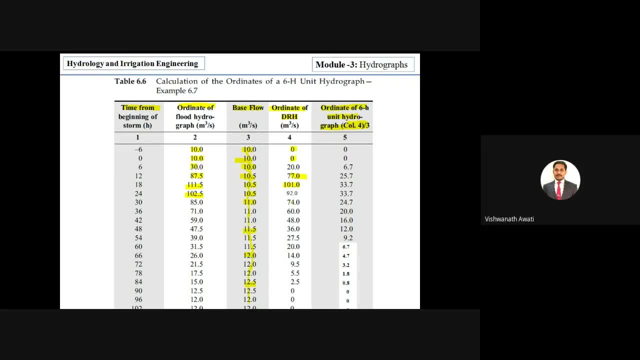 by subtracting ordinates of flood hydrograph by base flow, we will get these values right. So then we have to divide the values by subtracting ordinates of flood hydrograph by rainfall axis right, divided by 3, and we will see how we got this 3 right. it is a rainfall axis. 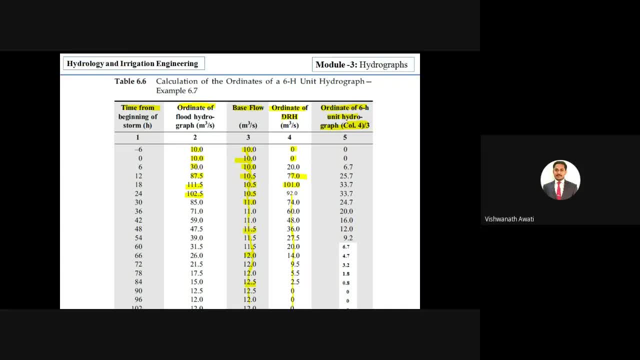 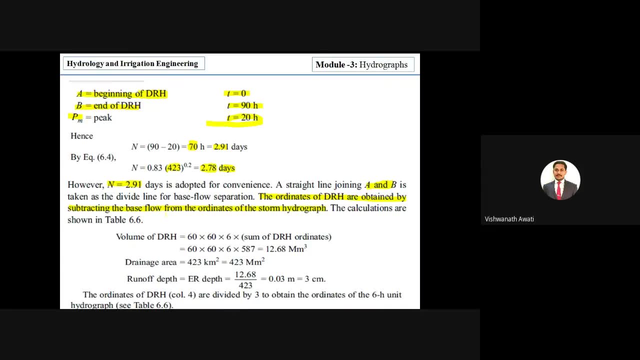 right as of now, we understood up to ordinates of direct runoff right. how to get this? by subtracting base flow for ordinates of flood hydrograph. So then we have to make the first calculation of volume of direct runoff hydrograph right. how to get volume of direct runoff hydrograph. 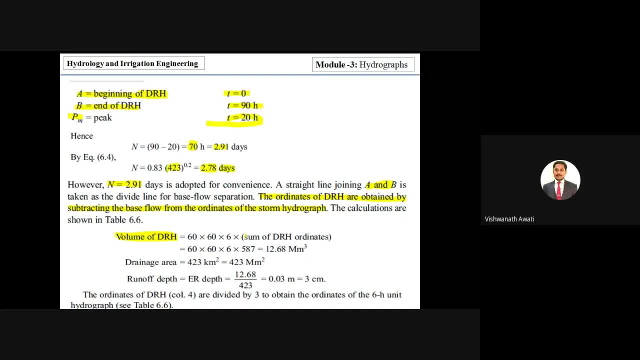 by 10.5 multiplying summation of direct runoff hydrograph ordinates. So here we got ordinates of direct runoff hydrograph and you make the summation of all this right column 4 and you will get value of 587, 587, right? So then this will be multiplied with the time. So time is in. 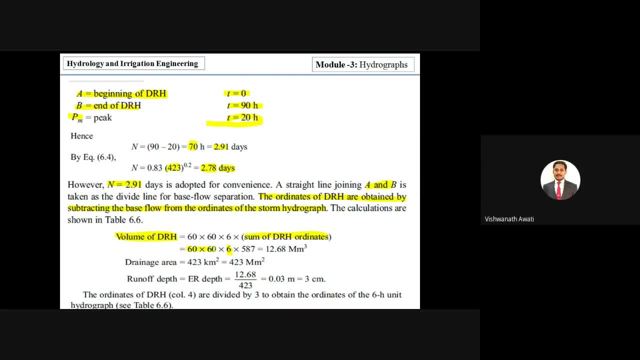 terms of r, but it is converted into centimeter. So then we will get the value of volume of direct runoff as 12.68 million meter cube. If we make the calculation of this, we will get 12.68 million meter cube. Next is: it is a very important and main important. 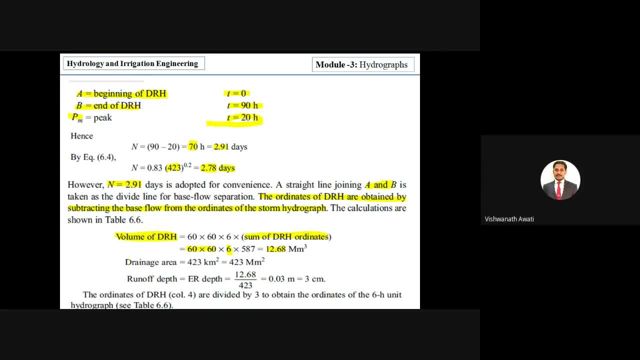 is summation of direct runoff coordinates. Next is drainage area. this is given in the problem, as this 423 kilometer square and it is converted into million meter square by because this is a given. Next, this is跑, which is twisted. however, it is converted to. million meter square because it is symmetric. and then also it is 8 and almost 15 얼마나 radius primeometer square. and wait, we have one. So first thing, think about it, draw back, because one Now, when you come to 따�� смог, it will start to go right. so, right in the middle, 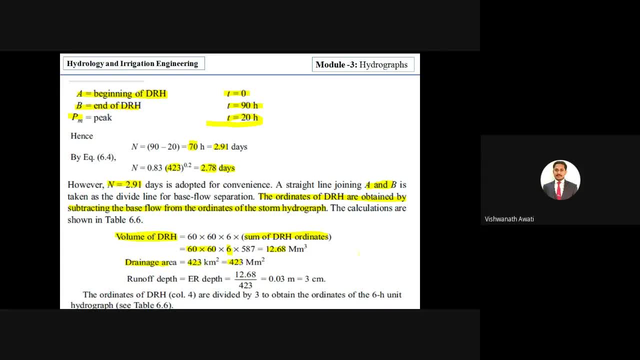 is in kilometer square and if you make, kilometer is 10 to the power 3 right, 10 to the power 3 meter right, 10 to the power 3 meter, but we have a square correct. so then it is what? 10 to the power 6 meter right, that is in terms of they have taken million right- 423 million. 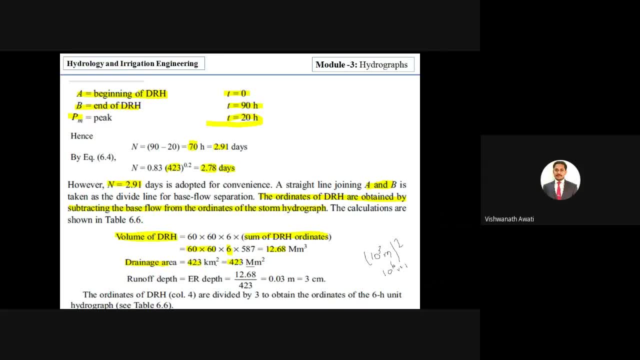 meter cube right. why? because it is in kilometer square and one kilometer is equal to thousand meters. 10 to the power 3 right and due to the square it will come to right. 10 to the power 6.. so then to get rainfall depth. it is very important right to get rainfall depth, excess rainfall. 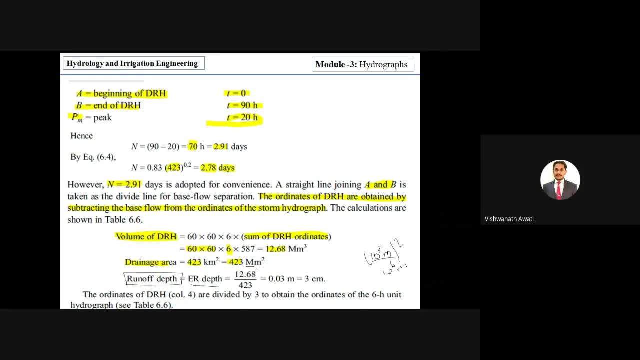 depth, right, uh, to get this, we have to get volume of direct runoff, that is 12.68, and area of the catchment, area of the drainage area. yeah then, and we have these values. if you calculate, we'll get point 0.03 meters, and if you calculate in terms of centimeter, we get three centimeter. 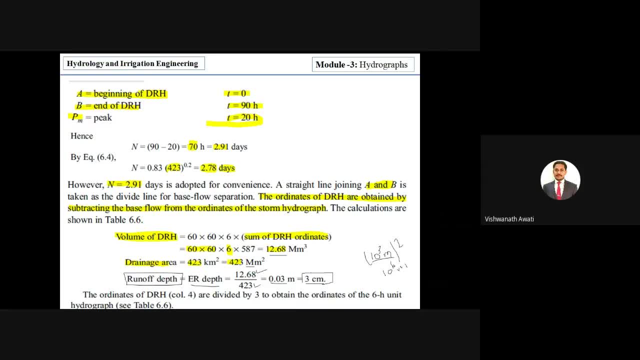 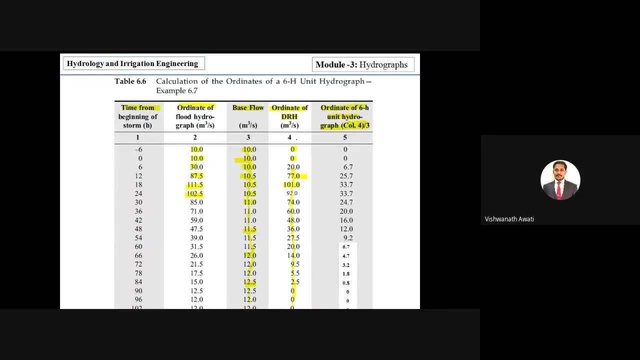 right and this three centimeter is rainfall access and this rainfall access is divided to column four of direct runoff hydrograph. then we get ordinates of six r unit hydrograph. so you can see, here we have a ordinates of directon of hydrograph. and if you make dividing of column four, 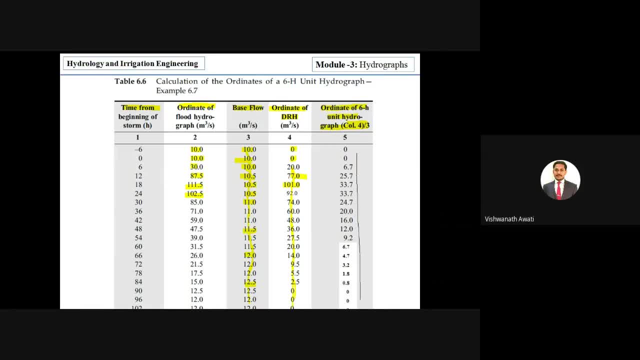 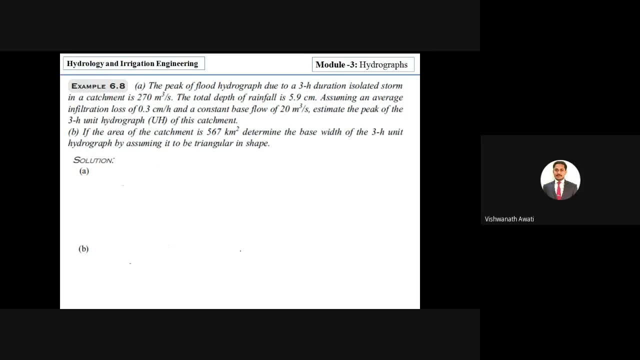 you will get ordinates of 6 r unit hydrograph. so these were final calculation, right, okay? so then we will go for next problem, right here. example: a peak flow, a peak of flood hydrograph due to 3 r duration. so here it is what peak of flood hydrograph due to 3r duration, how much is a? 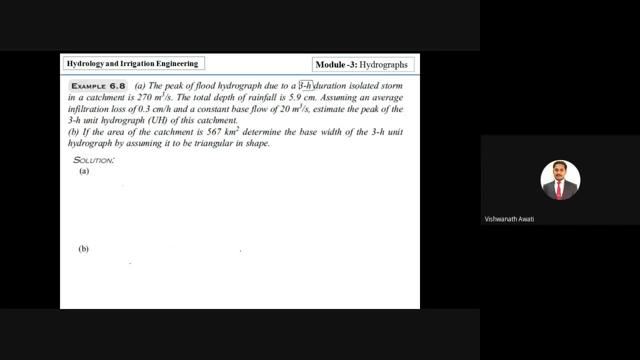 duration: 3 hour right. Very important Duration: isolated storm in a catchment is the peak flow hydrograph right. The peak flow hydrograph is 270 meter cube per second, right Of 3 hour duration. The total depth of the rainfall: the depth of the rainfall is 5.9 centimeter, Assuming. 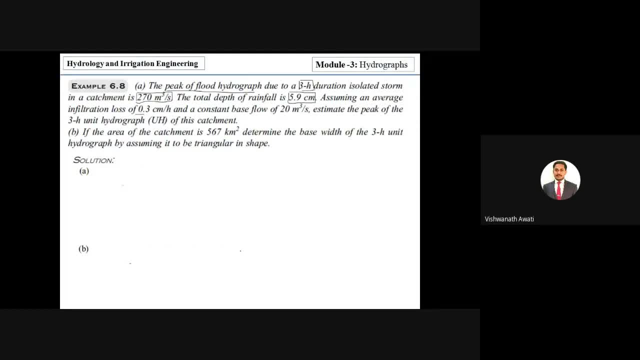 an average infiltration loss. the average infiltration loss is 0.3 centimeter per hour. and the constant base flow. here they have given constant base flow not varying 20 meter cube per second. Estimate peak of the 3 hour unit hydrograph: here they have given peak flow and we have to. 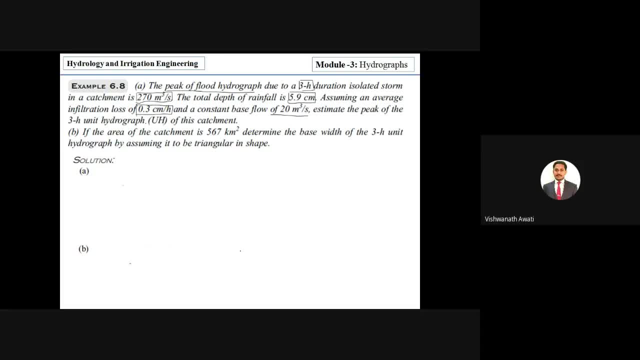 estimate peak of the 3 hour unit hydrograph right Of this catchment right And next is question B: If the area of the catchment is 567 kilometer square, determine the base width of the 3 hour unit hydrograph by assuming it is to be triangular in shape. 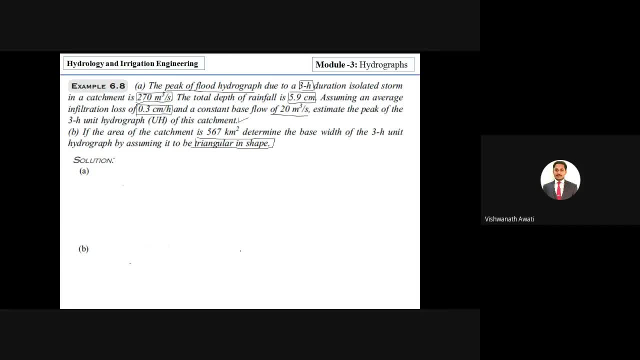 the triangular shape. It should be assumed in a triangular shape, See. first one is we have to estimate the peak of the 3 hour unit hydrograph right. And second one is we have to make the base flow width taken. base flow width, We will see one by one. So first one to calculate. 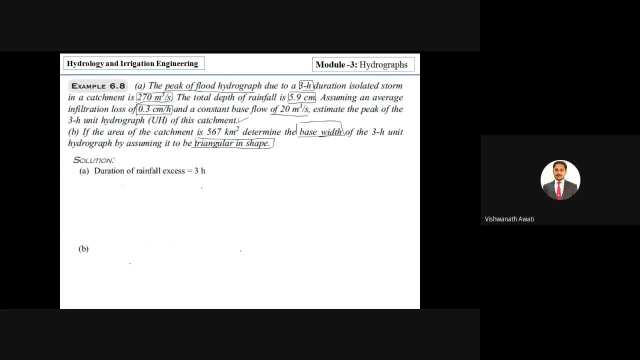 the peak of the 3 hour unit hydrograph right. Duration is 3 hour and total depth of the rainfall is 5.9 centimeter. it is given correct. So then even one more data: is loss 0.3 centimeter. 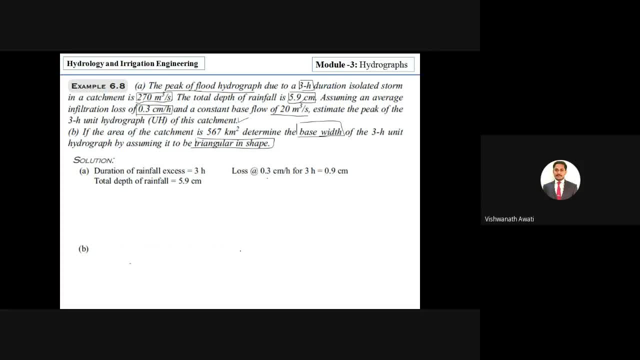 per hour, but totally how many hour? it is 3 hour right, And 0.3 into 3 is 0.9, correct In terms of loss, correct. So then the rainfall excess, right, It is what Rainfall minus. 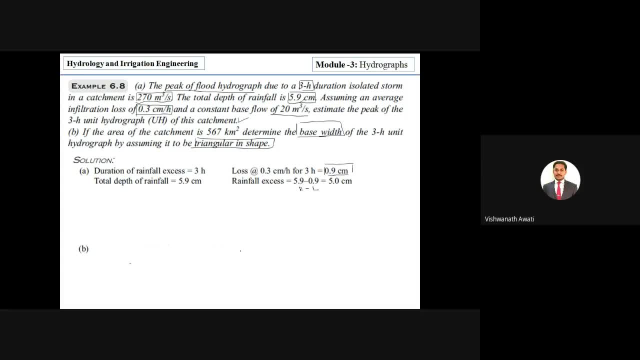 losses. Here we have a rainfall minus losses And we got a losses as 0.9.. And when you subtract 5.9 as a total rainfall depth minus 0.9, we will get rainfall excess as 5 centimeter. 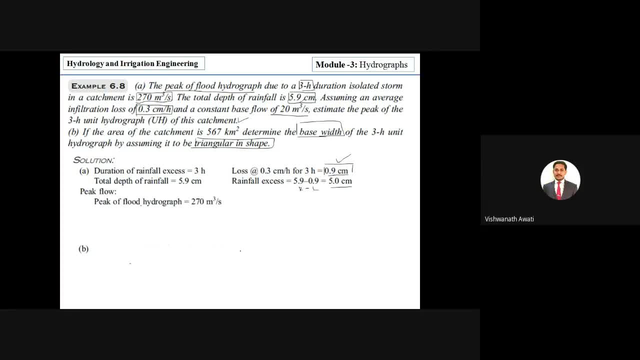 So next is peak flow calculation. So in that peak of the flood hydrograph is 270 meter cube per second, This is also given in the problem. Next is base flow is 20 meter cube per second. It is also given in the problem. Then we have to calculate the peak of the 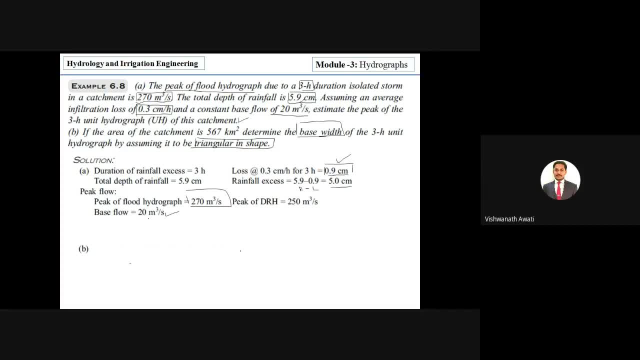 direct runoff hydrograph, that is 270 minus 20.. Because direct runoff hydrograph we will get, after subtracting base flow right, 270 minus 20, 250 meter cube per second. Next is peak of 3 hour unit hydrograph. We have a similar problem. We have a similar problem. 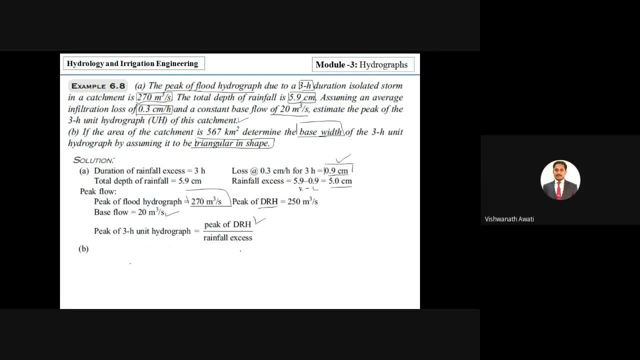 The sameэимсяple formula. peak of the direct runoff hydrograph, that is 250 rainfall divided by rainfall axis, that is 5 centimeter. So then 250 by 5, we will get 50 meter cube per second. This 50 meter cube per second is the peak point. flow, correct Peak flow. It is a first. 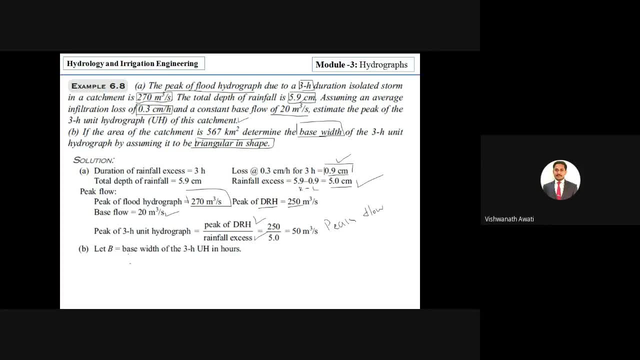 calculation requirement. Next we will go for second. that is peak point liquid flow. okay, That is peak flow÷÷thousandennes. go for second. that is base width calculation for 3R unit hydrograph for the same catchment, correct. 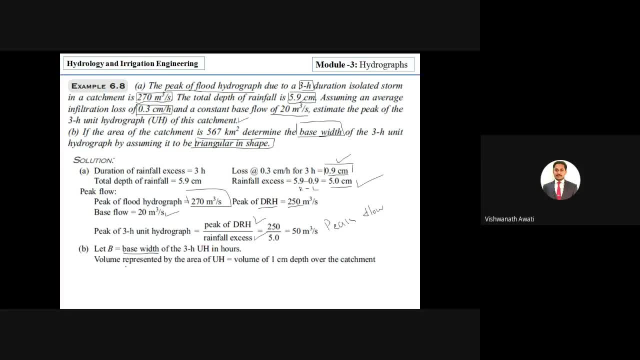 So here the assumption is the volume represented by the area of unit hydrograph. the area of unit hydrograph, correct, that is equal to volume of 1 centimeter depth over the catchment. So here it is. assumption is what volume represented by the area of the unit hydrograph. 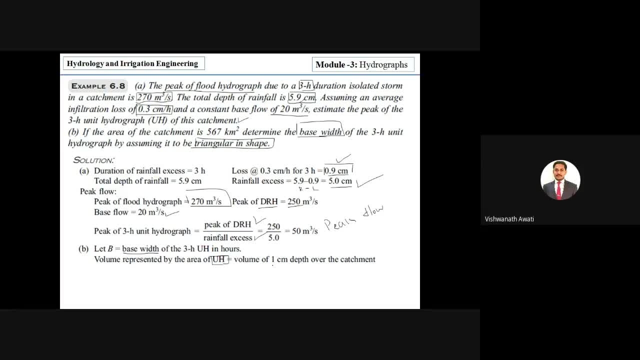 that is equal to volume of 1 centimeter, that is a unit depth over the catchment. So then the area under the unit hydrograph. how to solve this? by assuming it is a triangular. So here it is what hydrograph right and it is what triangular used, word to be triangular, correct. 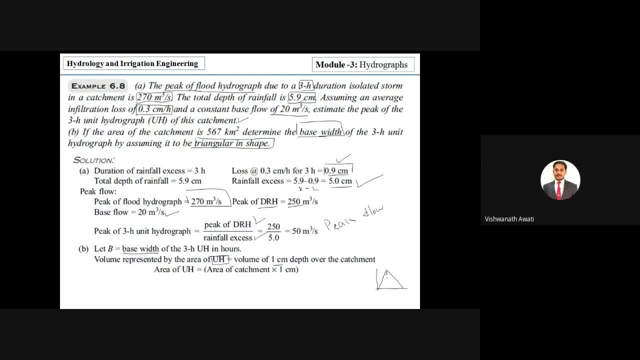 it is the starting point, it is the end point and we required peak point and we have a peak point. that is what? 50 meter cube, meter cube per second, correct? So then we have to calculate this base width as a right. So, as it is the area of triangular, then we have simple formula right, why? because it is. 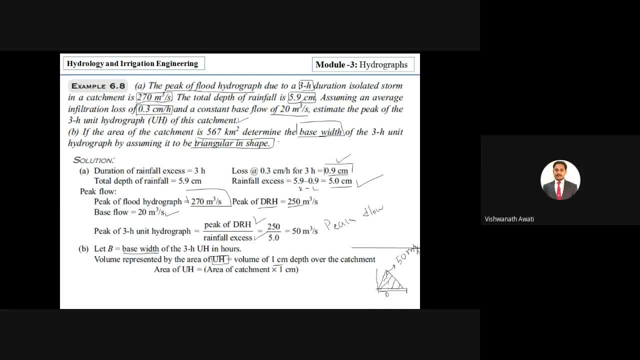 the area of unit hydrograph. and unit hydrograph is assumed to be triangular shape, correct? And we know the simple formula that is half base into height, correct? So it is half base is b and height is 50, because it is a, 50 meter cube per second and a meter cube per second and it is 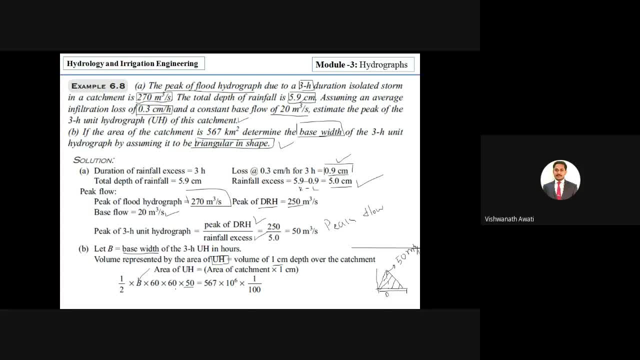 multiplied with a 60 into 60, correct, it will be converted into r, correct. So then, and it is area of the catchment, area of the catchment into 1 centimeter. So area of the catchment is, given it kilometer square, but it is, it is converted into, it is like a kilometer square and it is converted. 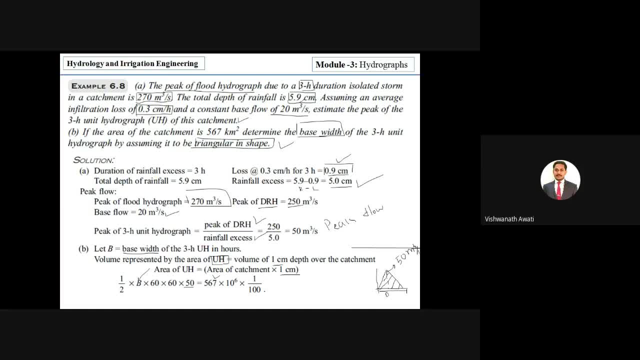 into meter, correct? And here it is a 1 centimeter. this is divided by 100 and means it is converted into meter and time is converted into hour, right? then it is unknown is only b, right, We can calculate b and we are getting the base flow width is 63 hours. 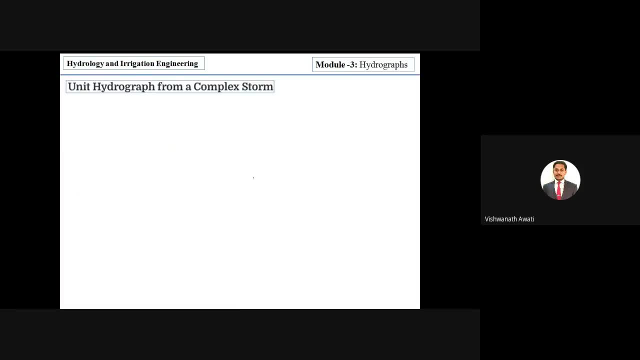 so two calculations are over. So next is the derivation of unit hydrograph from complex strom, and this is also not important in the exam point of view, but we will go through this Here. it is when suitable simple isolated strom are not available, the data from complex strom of the long. 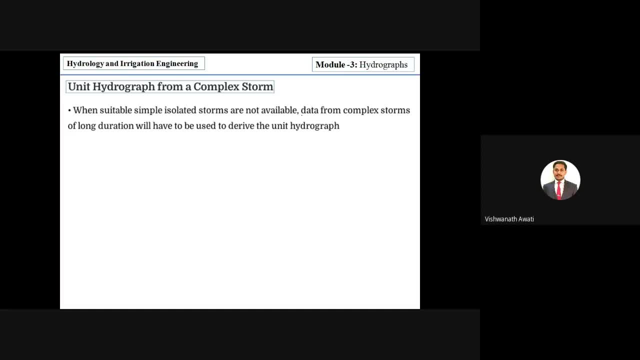 duration will have to be used to derive the unit hydrograph. So when we are not getting simple isolated strom, Then it has to be derived from a complex strom right to get unit hydrograph. but it has some problem. The problem is to decompose a measured composite flood hydrograph into its components of 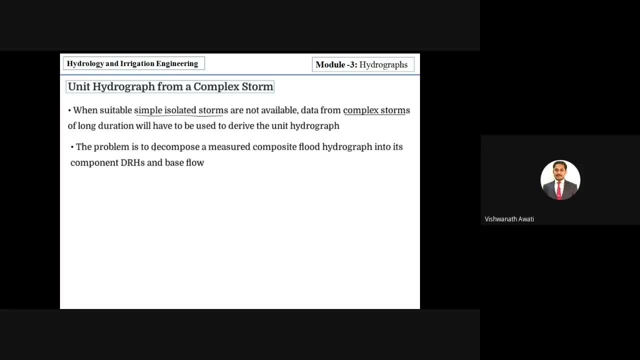 direct runoff hydrograph and base flow. It has some problem with the decompose of measure measured composite flood hydrograph And the common unit hydrograph of approximate duration is assumed to be exist. there is assumed to be exist of unit hydrograph. This is the inverse problem. 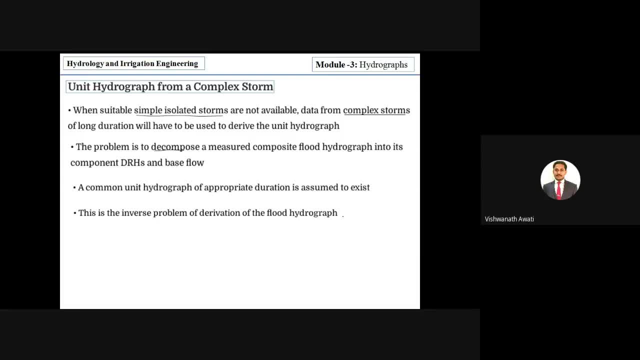 of derivation of flood hydrograph. So we made the derivation of flood hydrograph from the unit hydrograph and we are going with the inverse of same problem, right ok, Consider a rainfall excess made up of three consecutive duration of dr and excess rainfall values are r1,, r2, r3.. 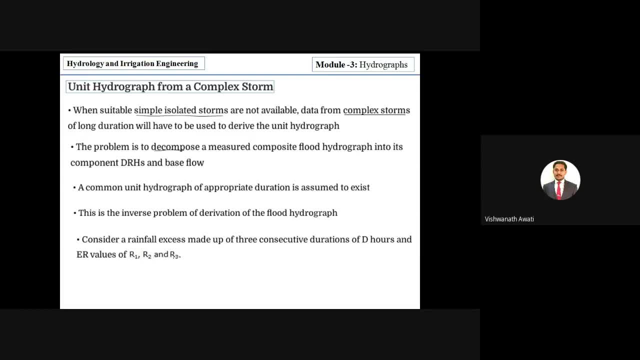 So what is the consideration of rainfall excess of three rainfall access of duration d and one rainfall is r1, second one is r2 and r3. of each d hour duration, Yes, one is 1d, 2d and 3d duration. Then, after base flow separation of the resulting composite flood. 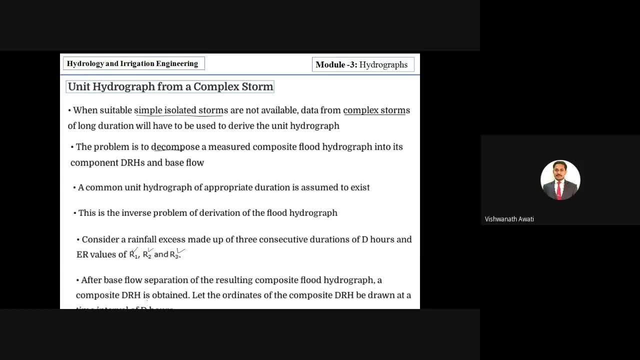 hydrograph. a composite direct runoff hydrograph is obtained by separation of see. here we have a flood hydrograph, and when you make the base flow separation you will get direct runoff hydrograph right. So then you can get composite direct runoff hydrograph. Let the ordinates of the 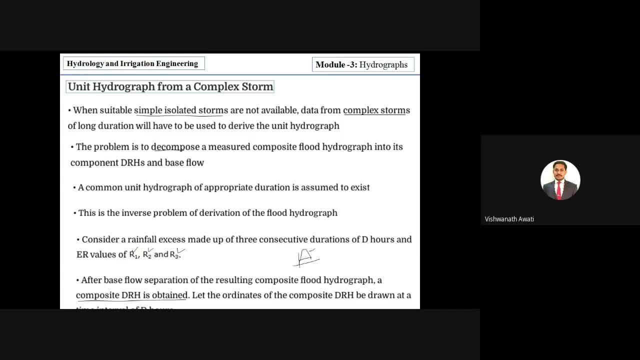 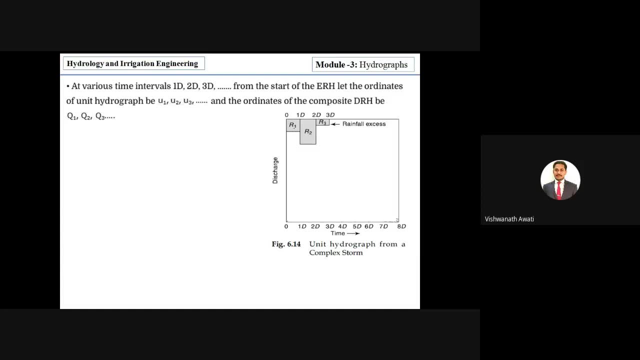 composite direct runoff hydrograph to be drawn at a time interval of dr's right, the dr's. So then, as I told, there is a consideration of 3 excess rainfall of r1,, r2, r3 with respect to dr's right. Then at various time interval- 1d, 2d, 3d from the starting point of excess rainfall. 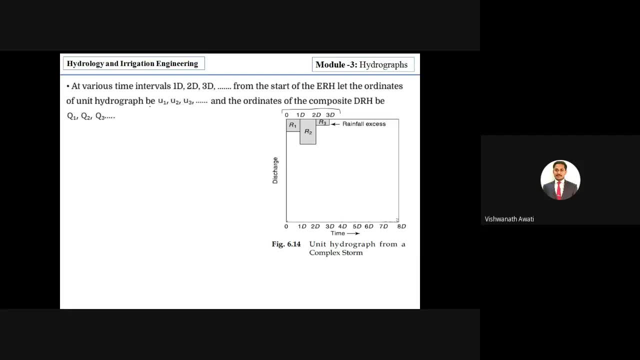 hydrograph. let the ordinates of unit hydrograph to be u1, u2, u3 and the ordinates of composite direct runoff hydrograph to q1, q2, q3.. So here we have to understand. time duration is 1d. 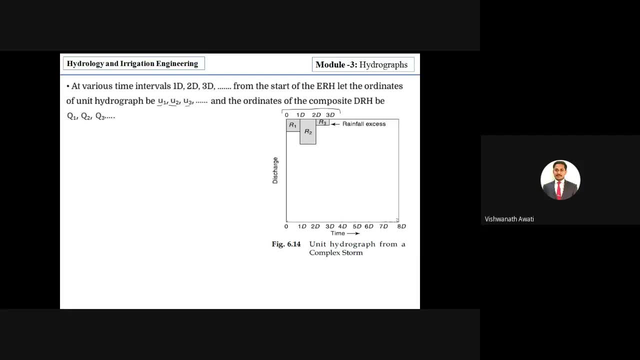 2d, 3d, and the ordinates of unit hydrographs are u1, u2, u3. Then ordinates of direct runoff hydrograph is q1, q2, q3.. Then how to calculate, how to get like no relations between ordinates of direct runoff hydrograph and unit hydrograph. So 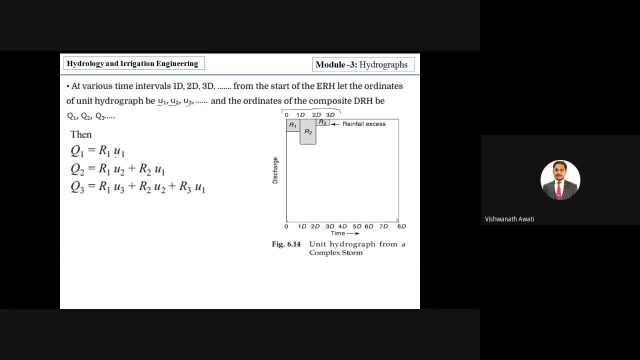 here is a simple formula of inverse method of flood hydrograph derivation, that is, the relation between: like no ordinates of direct runoff hydrograph is q1, that is equal to r1, into u1. So it is rainfall excess. 1, multiplied by it is ordinates of unit hydrograph and, if you observe, we have a formula like this: 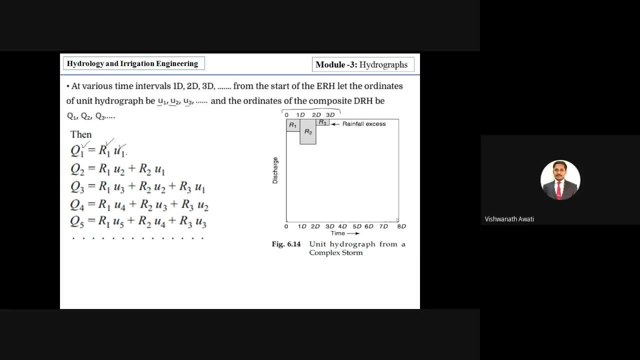 r1, r1, r1, r1. it will be same, but it is changing with unit hydrograph ordinates. it is u1, u2, u3, u4, u5.. Again, it will be taken like no lesser than u, like no, which one you use in the first.